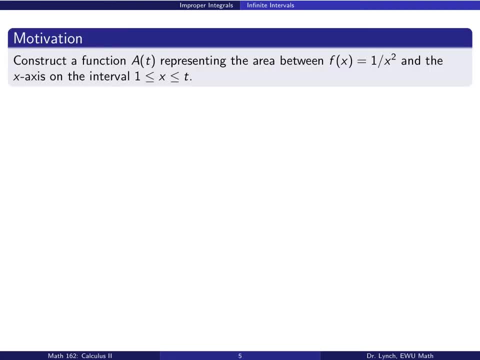 So start off with the expression. This is the idea of an infinite interval. Let's go ahead and construct a function a of t that represents the area between the curve 1 over x squared and the x axis on the interval from 1 to t. 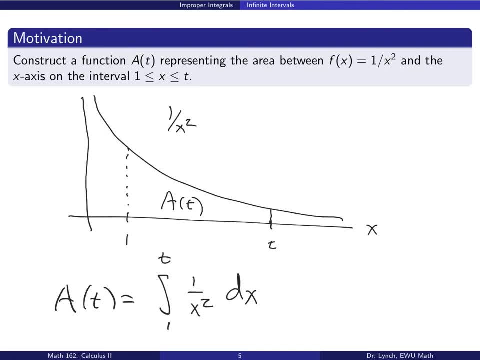 So pictures are nice. Let's draw a picture first. So here's a graph of our function: 1 over x squared. Here is the area under the curve between 1 and some unknown value, t, and we know how to express this as an integral. 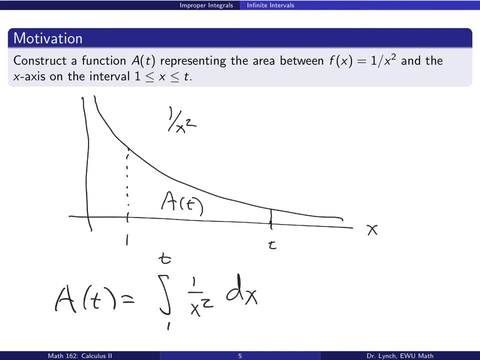 And in fact in this case we can go ahead and evaluate the integral. It's not so bad to do just using the fundamental theorem of calculus with the variable endpoint t. In this case we see that that area integral evaluates as 1 minus 1 over t. 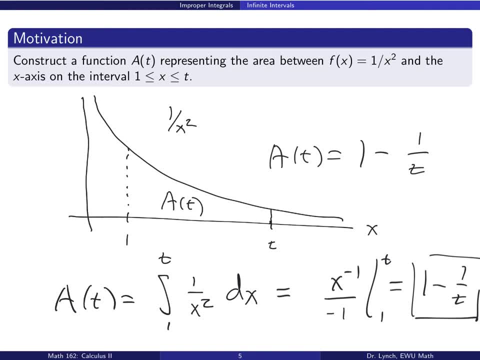 So you can imagine, for instance, if t was 2, the area a of 2 would be 1 half, and if t is 3, the area would be 2 thirds, and if t is 4, the area would be 3 fourths. 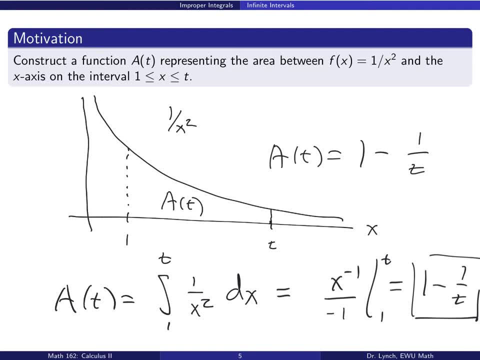 and if t was 2, the area would be 10, the area would be 9 tenths, and so on and so forth, And in fact, one thing we can think about doing is think about letting t be arbitrarily big, And in fact, 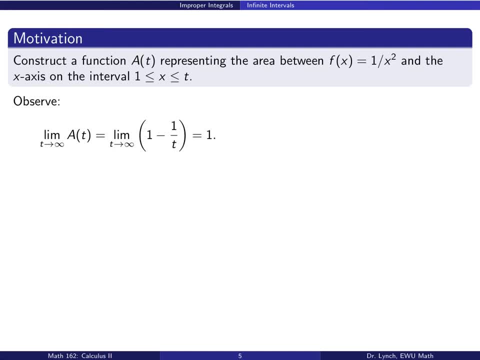 the limit, as t goes to infinity, of a, of t is 1 minus 1 over t as t goes to infinity, of course, and that limit is 1.. So this, in fact, is how we understand an infinite interval on our integrand. 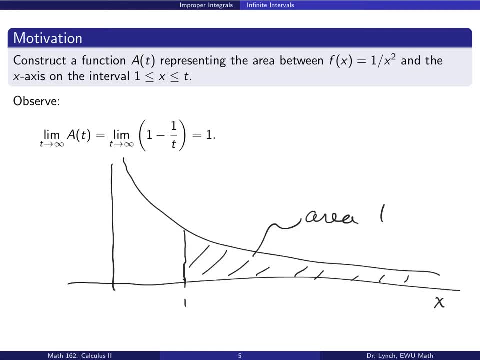 We understand that the integral of t is 1 over t, and that's true. So we've got this interval. So we've got the interval. the area under the graph of 1 over x, squared from 1 to infinity, is finite with area 1.. 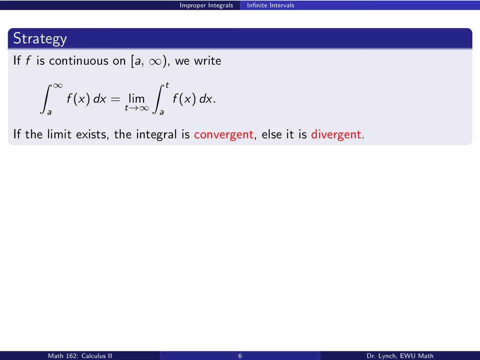 in general, this is how it looks. if we have a continuous function and we wish to evaluate an integral with an infinite limit- from a to infinity- what we do with that integral is write it as a finite integral, first from a to t, and then take the limit as t goes to infinity. if 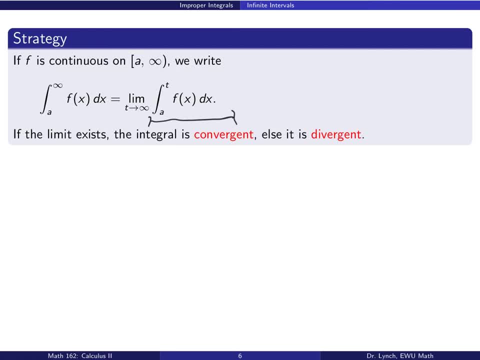 the limit exists, we say the integral is convergent, otherwise we say it is divergent. here's an example. let's determine whether the integral is convergent. if so, give its value. in this case, we'll have the improper integral, from 1 to infinity, of 1 over x, dx. 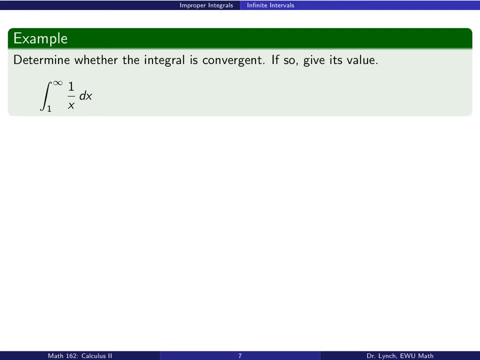 this is something, again, that we'll write as a finite, an integral on a finite interval, and then let the end point go to infinity. so this is the first step: expressing the integral on the infinite interval as the limit of an integral on a finite interval. now we can know how to evaluate. 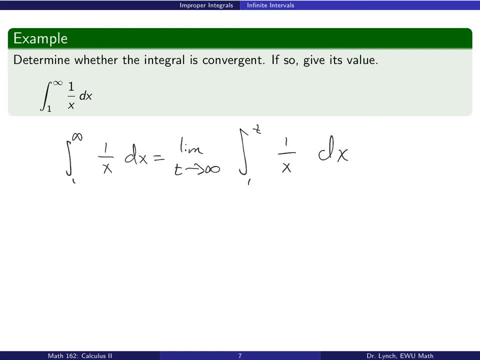 this definite integral, we can just express it as the natural log function and use the fundamental theorem of calculus to plug in the limit. so at the end of the day here, what we end up with is the solution that you answer is that the integral is divergent from a double-sub-limit limit. 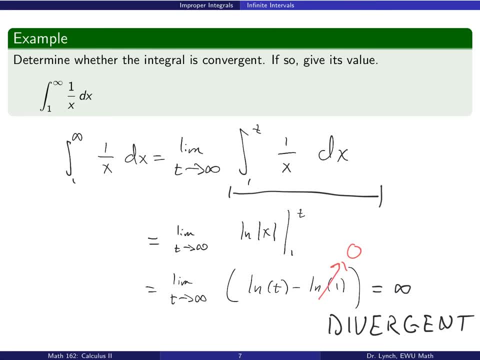 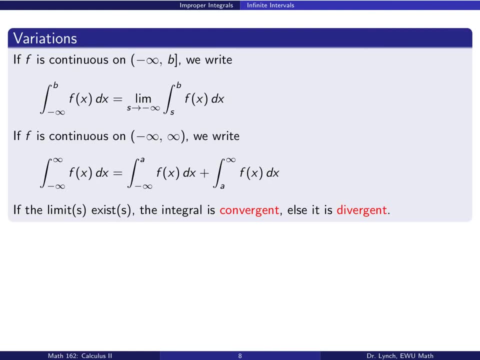 of t verdade. okay, so again, uh much, let's do another example. Sorry, before another example. we also could have an infinite limit to minus infinity, And we could also have a doubly infinite interval which we break up into singly infinite intervals. Okay, so, both of those things are possible. Let's go ahead and have a. 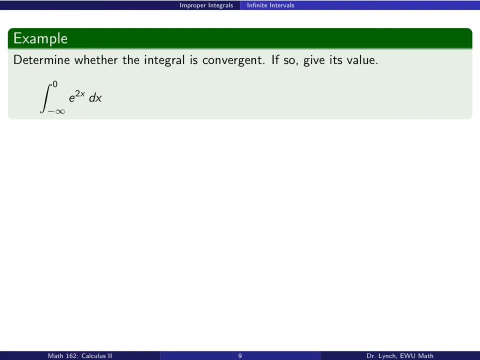 look at some more examples. Here's another example. Let's have a look at the integral from minus infinity to zero, of e to the 2x dx. So again, we'll write this as the limit of an integral on a finite interval. So again, here's the first step, expressing the improper. 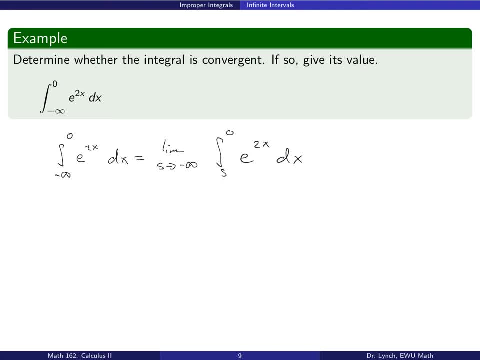 integral as the limit of an integral on a finite interval. when we can understand, We can now go ahead and evaluate this finite interval Vol with fundamental theorem of calculus and then take the limit to see what happens. In this case we see that the integral evaluates as 1 over 2 e to the 2x between s and 0. 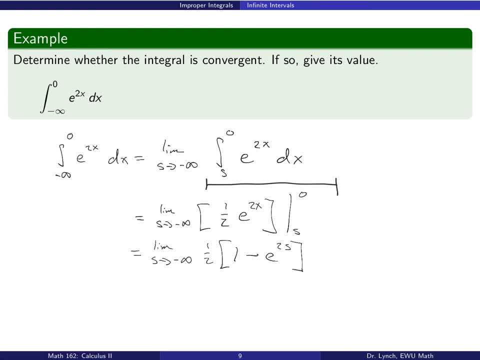 We plug in 0,, we get 1.. We plug in s, we get e to the 2s, And as s goes to minus infinity, this exponential part goes to zero. So we, So we can see that we're left with 1 half. The integral is convergent and its value is 1 half. 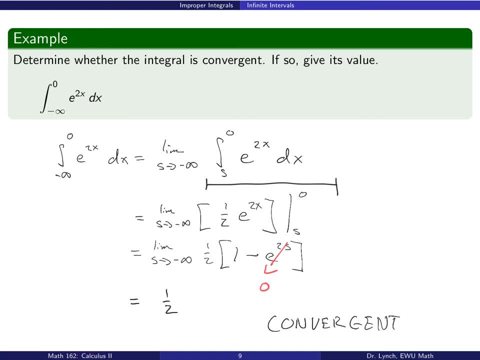 Okay. so again, because the limit exists, we say that the integral is convergent and takes on the value of the limit, which in this case is 1 half. Okay, let's do another one. Go ahead and have a look at the doubly infinite interval, from minus infinity to infinity, of 1 over x squared. 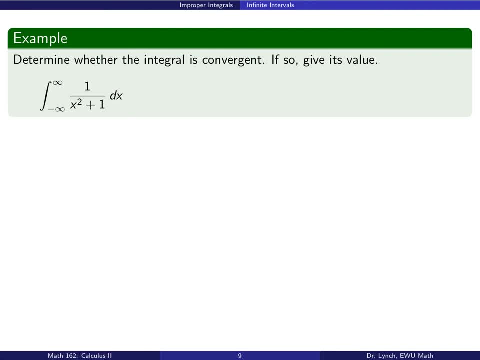 Plus 1 dx. So again in this case we'll express this as the limit of two singly infinite intervals. So here is that integral on a doubly infinite interval, expressed as two singly infinite intervals. Having a look at the first one, we see that we can write it as limit as s goes to minus infinity, of the integral from s to 0 of 1 over x squared plus 1.. 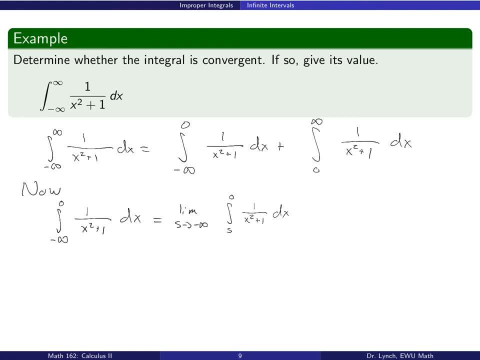 And of course we can evaluate this. We can write the integral using fundamental theorem of calculus and then let the limit as s goes to infinity. We'll see what we get there. Of course, 1 over 1 plus x squared has an antiderivative of arctan of x. 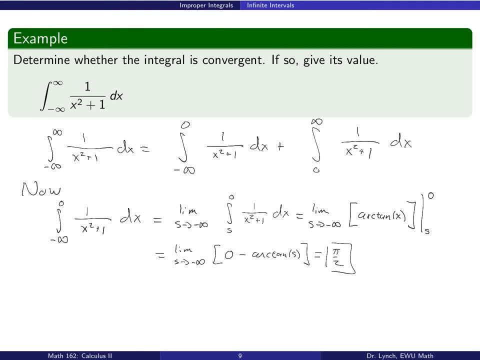 We can evaluate that at 0 and s, And as s goes to minus infinity, arctan goes to minus pi over 2.. With the additional minus sign we see that the integral here is pi over 2.. It works the same way on the interval from 0 to infinity. 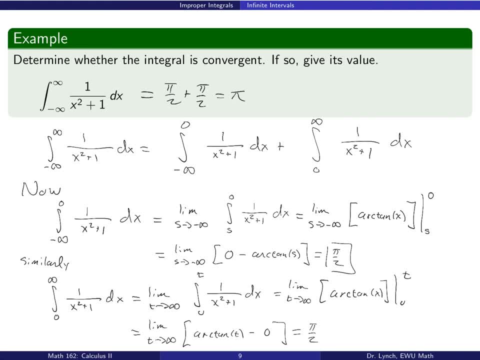 In the case of the integral from 0 to infinity, we see that it can be evaluated as the limit, as t goes to infinity, of the integral from 0 to t of 1 over x squared plus 1.. Of course, again, the antiderivative is arctan. 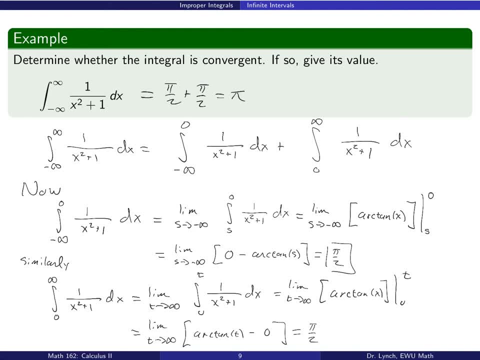 Plug in t and plug in 0 and take the limit as t goes to infinity, The value of that integral is pi over 2.. The original integral is continuous. The original integral is convergent And in this case we see that its value is pi over 2 plus pi over 2, so pi. 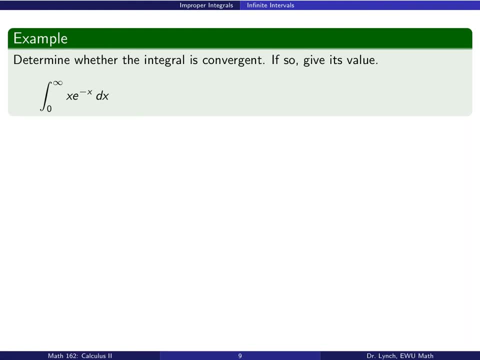 Sometimes improper integrals require integration by parts and L'Hopital's rule. So this is an example of that. So we start off expressing our improper integral as the limit of an integral on a finite interval. Use integration by parts with u equal to x and dv equal e to the minus x, dx. 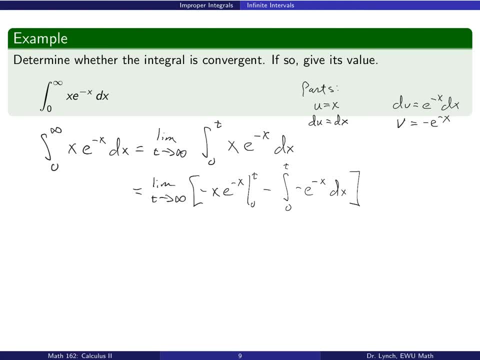 Go ahead and evaluate the new integral resulting from that integration by parts, And then we'll take the limit as t goes to infinity. So, after using the fundamental theorem of calculus, plugging in the limits of t and 0, we end up with the limit, as t goes to infinity, of the quantity. 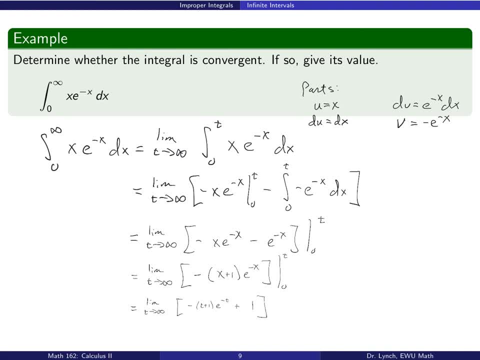 So that's t plus 1 times e to the minus t, all plus 1.. Now of course here's a limit that we can't evaluate right away. So we'll go ahead and sort of do that on the side And at the end of the day we'll find that our integral is convergent with value 1.. 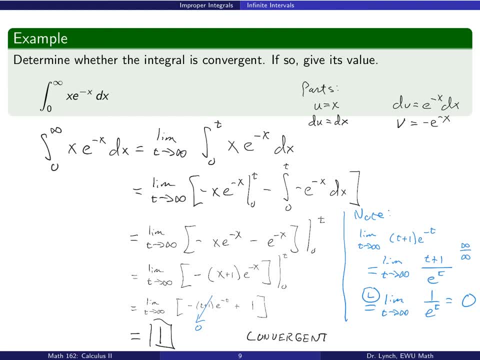 So here's our evaluation of the limit. using L'Hopital's rule, We can see that t plus 1 times e to the minus, t goes to 0 as t goes to infinity, giving us the value of 1 for our convergent integral. 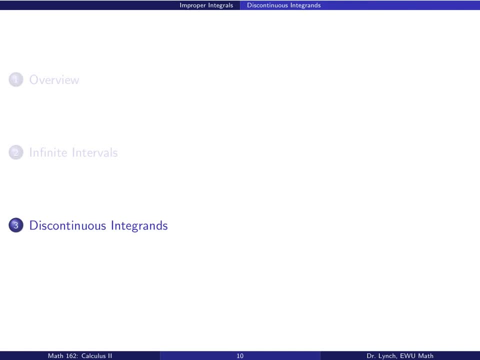 Okay, the other thing that might happen is there might be a discontinuous integrand So we'll go ahead and sort of frame that the same way by rewriting our improper integral with a single discontinuity as an integral on a finite interval with no discontinuities. 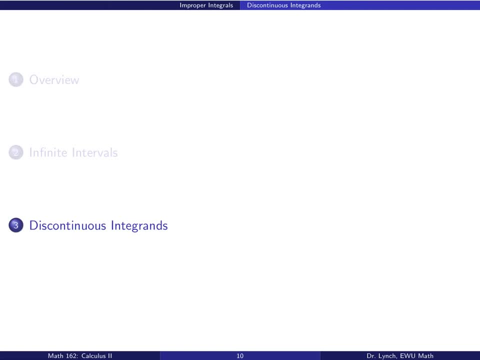 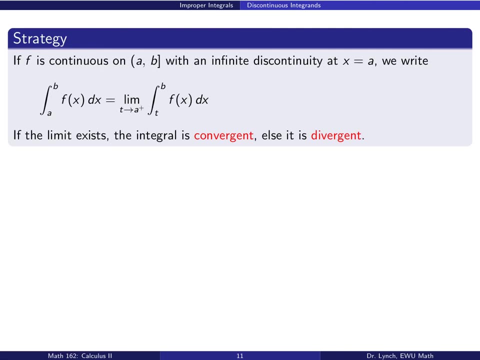 and then using the limit to push out to the point of discontinuity. So here's the first flavor. If we have a function f that's continuous between a and b, except with an infinite discontinuity at a, we'll go ahead and express our integral from a to b, of f, of x, dx. 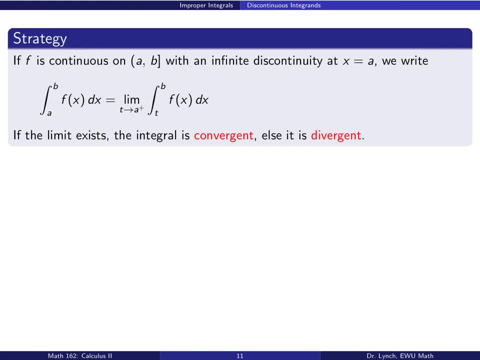 as the limit, as t goes to a from the right side, the integral from t to b, of f, of x, dx, and if the limit exists, again, we'll say that the integral is convergent. Okay, so an example of this type of an integral. 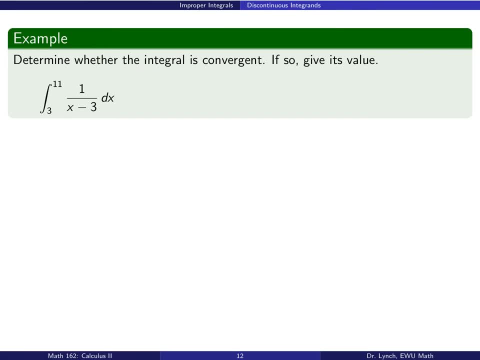 Let's go ahead and have a look at the integral from 3 to 11 of 1 over x minus 3 dx. So of course, here we can see that our integral, our integrand rather, is discontinuous. at the endpoint x equals 3.. 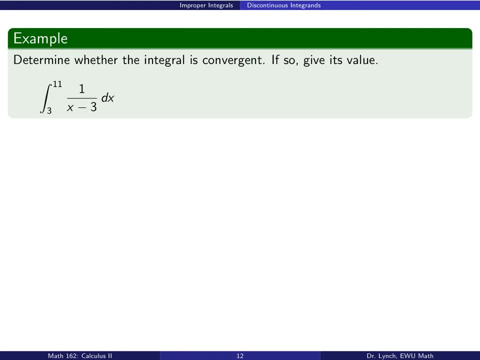 Go ahead and express this using a different interval and a limit. Okay, so again, here is that improper integral, rewritten with a limit and a finite interval. We can evaluate our integral on the finite interval using fundamental theorem of calculus and then go ahead and take the limit as t goes to 3 from the right. 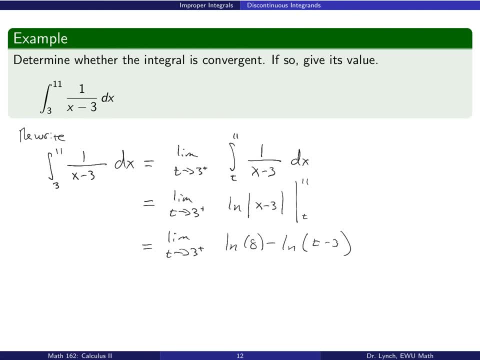 So we see, of course, that we're left with the limit, as t goes to infinity, of the natural log of 8 minus the natural log of t minus 3.. And sorry, I misspoke The limit as t goes to 3 from the right of the natural log of 8. 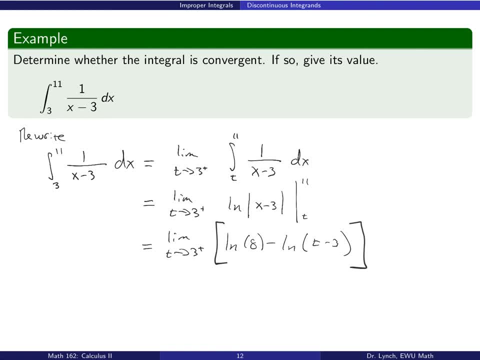 minus the natural log of t minus 3.. Now, of course, as its argument goes to 0,, the natural log goes to infinity. So we can see that the value of this limit is infinity. Since that limit is infinity, we say that the integral is divergent. 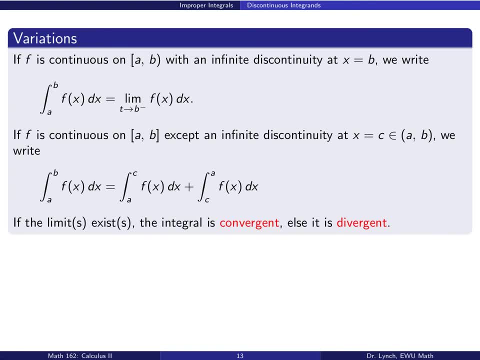 Two other things might happen with a discontinuous integrand. It might be that the discontinuity is at the other endpoint, like we see here, Or it might be that the discontinuity is in the middle. And if the discontinuity is in the middle, 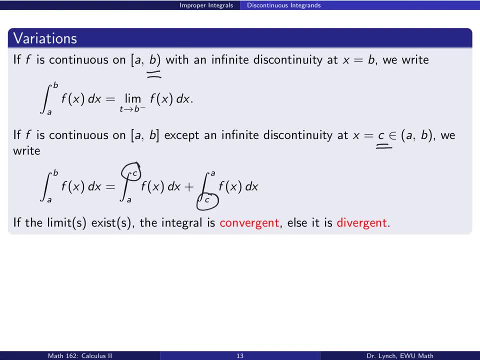 we can break it up into an integral from a up to that discontinuity and an integral from c, And this should be a b, not an a. And again, if limits exist, then we say integral converges. There should be an integral sign here. 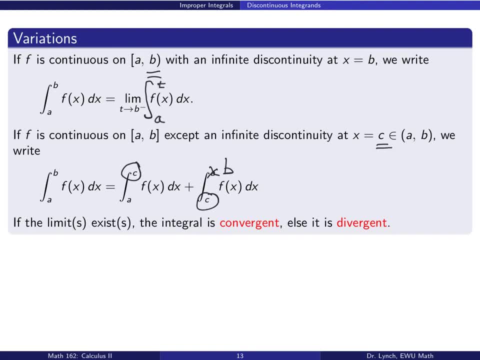 I'm not exactly sure what happened to that. And if the limits don't exist, then we say that the integral is divergent. OK, one sort of final example here. Let's go ahead and have a look at the integral from 1 to 10. 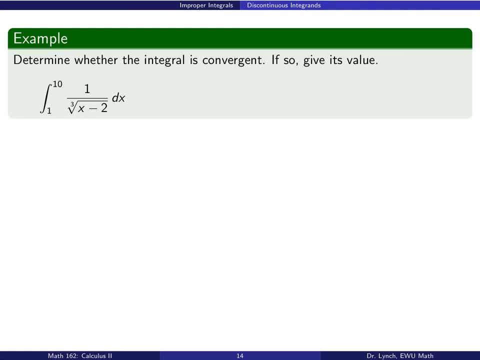 of 1 over the cube root of x minus 2 dx, We can see that the integrand is discontinuous at x equals 2.. So we'll go ahead and break this up by integrating from 1 to 2 and then integrating from 2 to 10.. 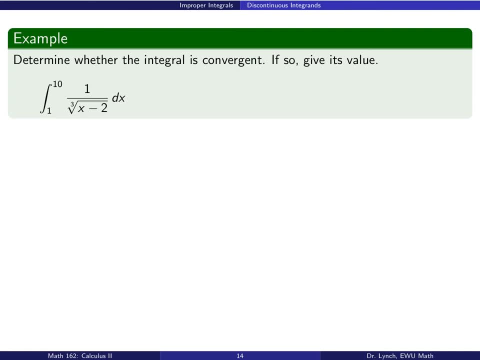 And then we'll see what happens in each of those cases. So here's our original integral on the interval from 1 to 10, broken up into two different integrals: one from 1 to 2, the other from 2 to 10.. 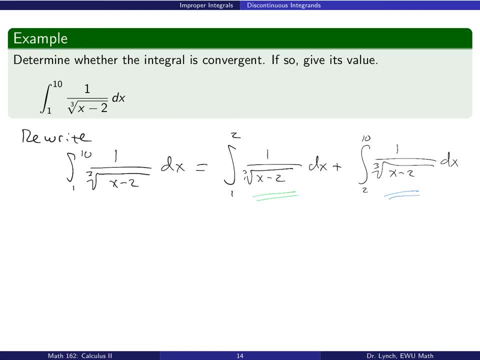 And we'll go ahead and examine those individually. now that one has a discontinuity at its upper limit of integration and one has a discontinuity at its lower integral interval of integration, I'll leave the u substitution to u, but we can see that the integral from 1 to 2. 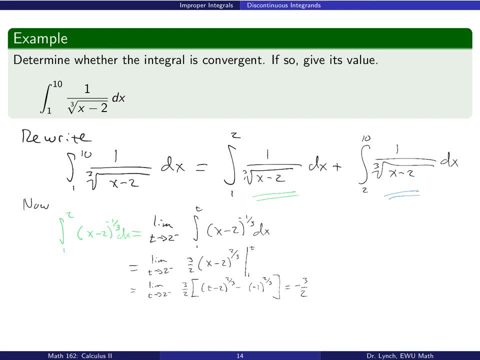 of x minus 2 to the minus 1 third. power dx can be evaluated by having a look at the limit as t goes to 2 from the left, the integral from 1 to t, of x minus 2 to the minus 1 third. 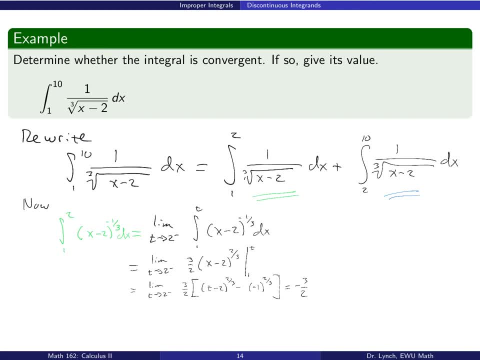 And at the end of the day here what we get is negative 3 halves for the value of the integral. The other integral turns out similarly And again, I'll just leave that as an exercise for you. OK, in this case we see that the value of the blue integral 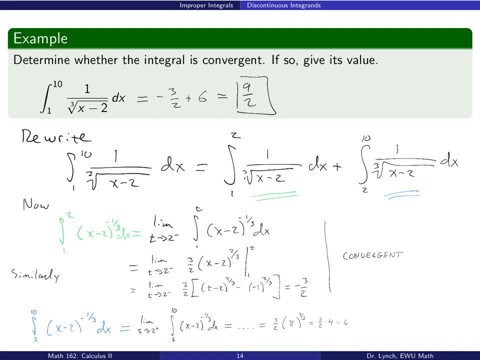 is the limit as s goes to 2 from the right, the integral from s to 10 of x minus 2 to the minus 1 third power, And I'll leave it to you to find that that value is 3 halves times 8 to the 2 thirds. 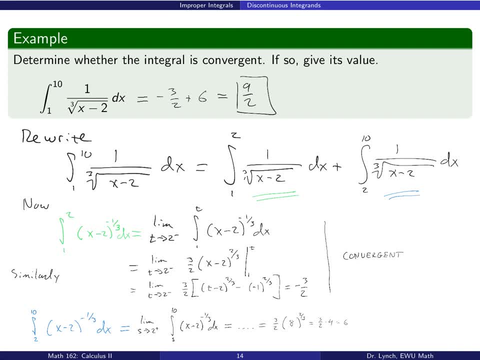 Of course, 8 to the 2 thirds is just 4, so the value in this case turns out to be 6.. This gives us, at the end of the day, a convergent integral, And the value that that integral takes is minus 3 halves plus 6,. 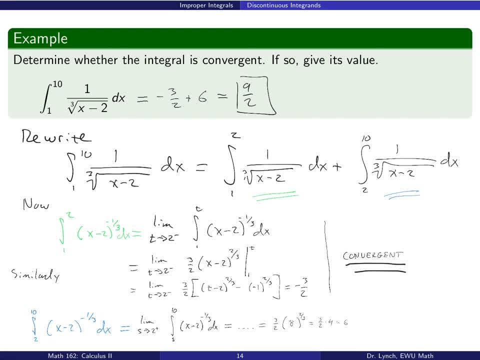 which is 9 halves. OK, folks, Hope you've enjoyed this video on improper integrals. Have a great day and we'll see you next time. Bye-bye.